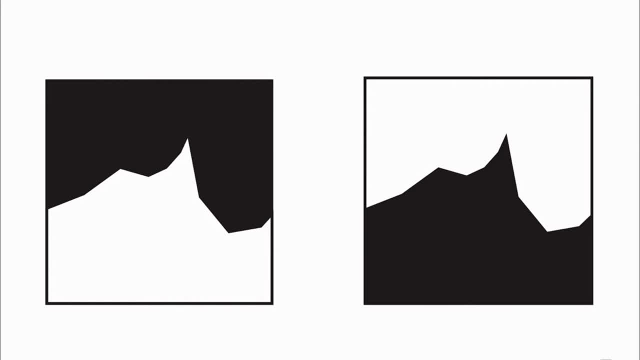 wondering if the corollary might be wrong. So, for example, if a large star in the world is a load of bears and a big space object, the bottom portion of whatever it is that you're looking at. so in this case we're looking at an area chart. the bottom is always perceived as being the figure meaning. 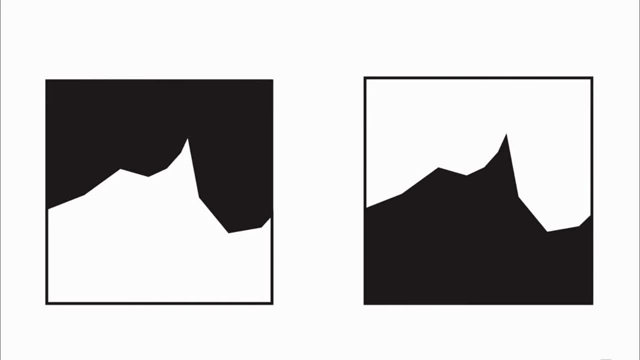 in the foreground and the top is the background, no matter what the color. If someone were to look at the area chart on the left, they're going to perceive the white as being the data and the black as being the background, And the same thing on the right-hand side: the black would be the data and the white 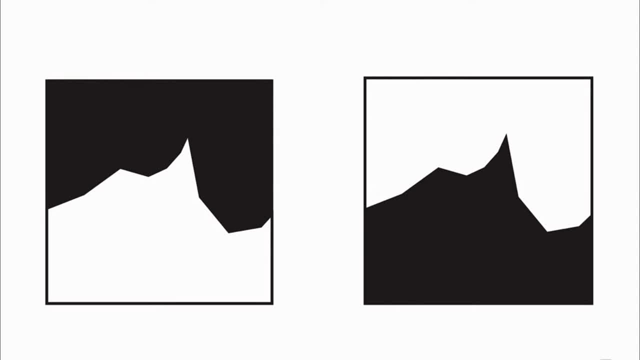 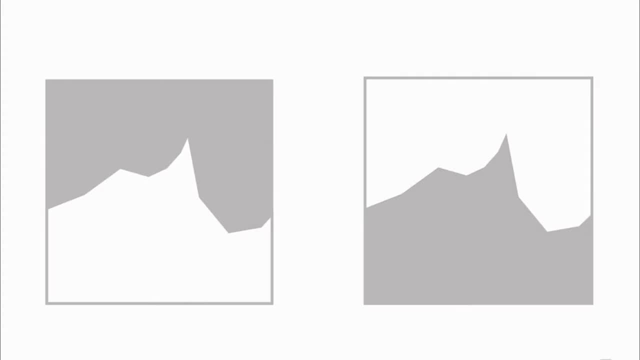 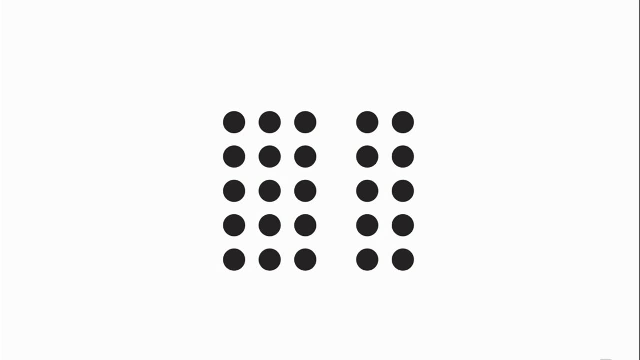 is the background, So you can't rely on color or contrast or anything other than bottom versus top. It's an important principle to understand. The next gestalt principle to talk about is proximity: When you have items next to each other or near each other. in this case, we have three. 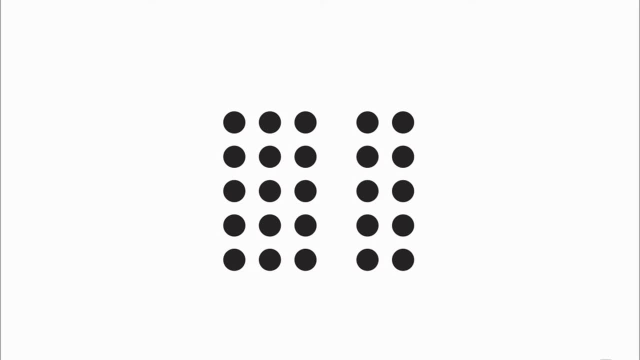 columns of dots on the left and two columns of dots on the right. they are perceived as being grouped and therefore similar and together. One will immediately sense that all the dots on the left-hand side are together and with each other, Yet separate from the two columns of dots to the right. 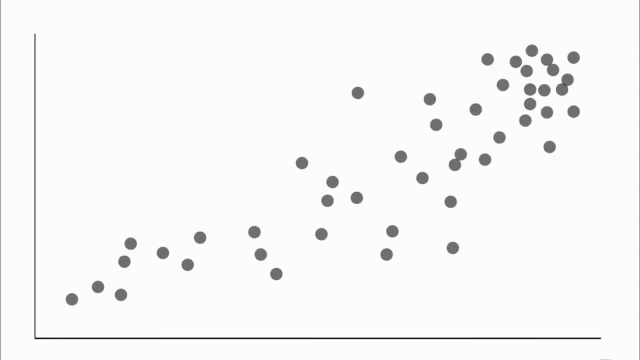 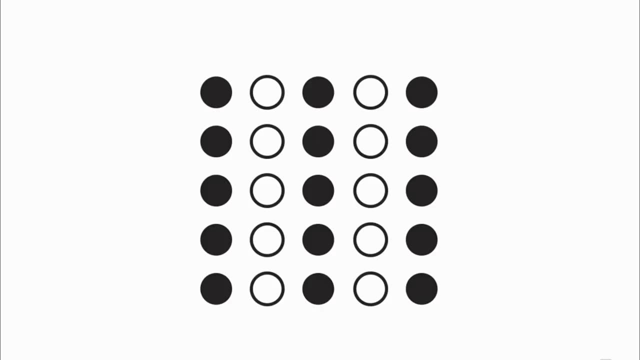 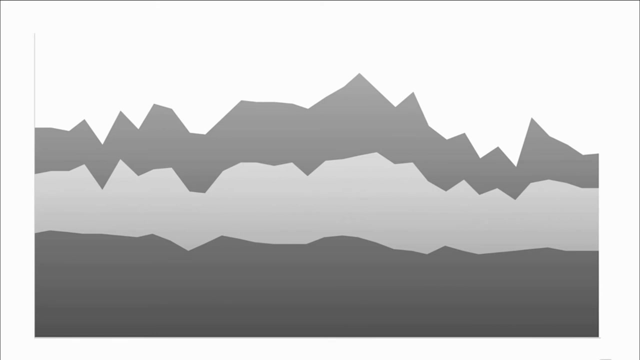 Proximity is one reason why we recognize patterns in a chart like this scatter plot. The next principle is called a similarity. Objects that are similar- the black dots- are different from the other objects- the white dots- straightforward. The similarity of things makes us categorize them, whether the similarity is in shape or 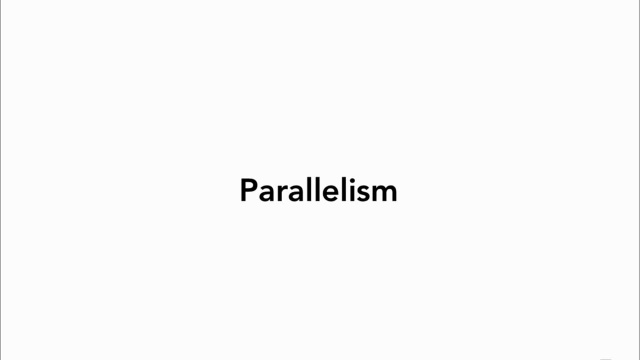 size or color. The next principle is called parallelism. The idea here is that when you have two dots on the left and two dots on the right, they are separated. When you have things in parallel, like the three lines in the middle, we assume that. 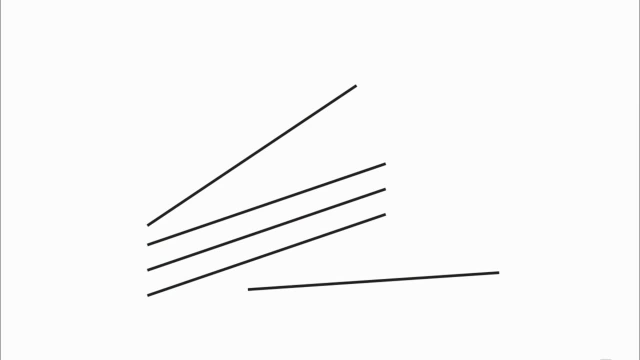 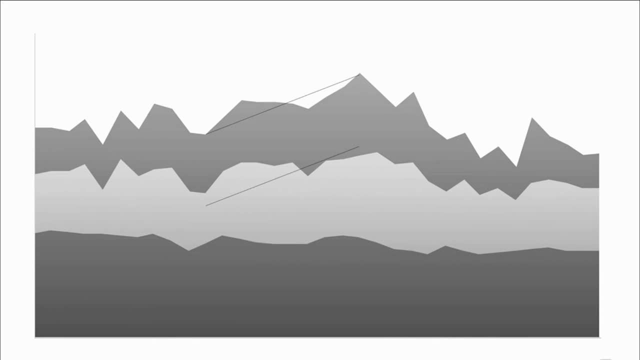 they're together and different from the other objects that aren't in parallel. In data visualization you might see patterns, For instance the overall trend lines for these different portions of this area chart. we see that parallelism and make judgments about these shapes because of that aspect. 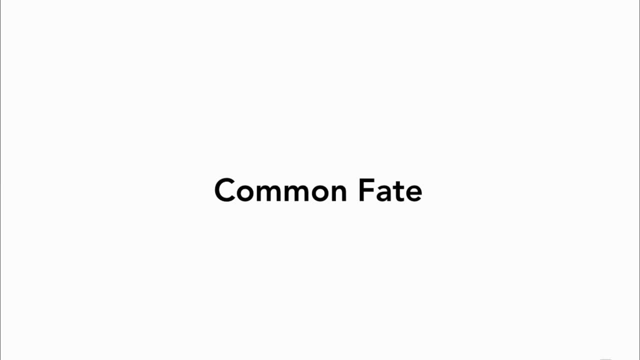 of the shape. The next principle is called common fate. Here you have a bunch of dots and there's no discernible pattern. But as soon as they start moving they become parallel. You can see that these dots have a common fate. 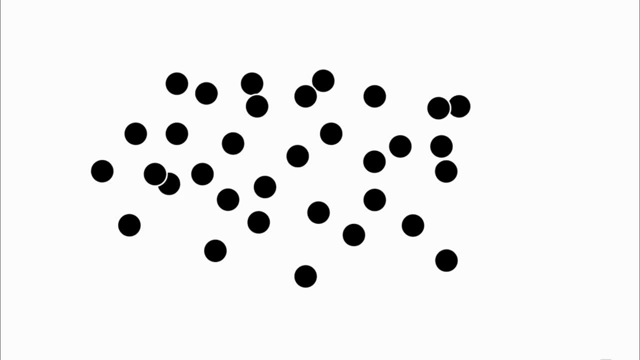 They're all moving in the same direction, so you can tell that they belong together. The ones that are moving are one group and the ones that aren't moving are in another group. That's common fate. Of course, you can see this in animated visualizations or interactive visualizations, where you have 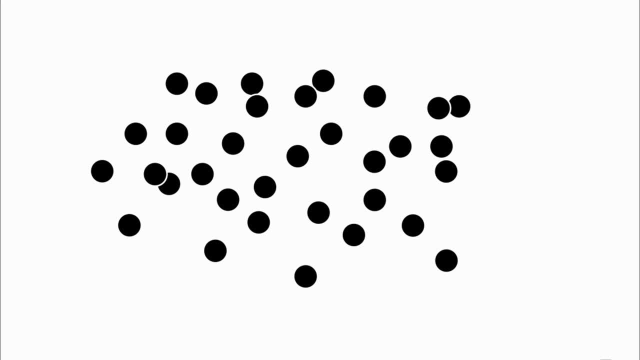 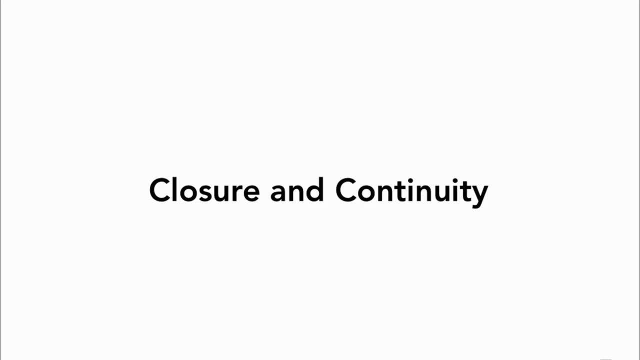 a rollover effect. You won't see this in static visualizations. There are the principles referred to as closure and continuity. These are interesting, although they're less relevant specifically for data visualization, but they play a role in really all design. The first idea here is closure: the fact that we see things that aren't there. 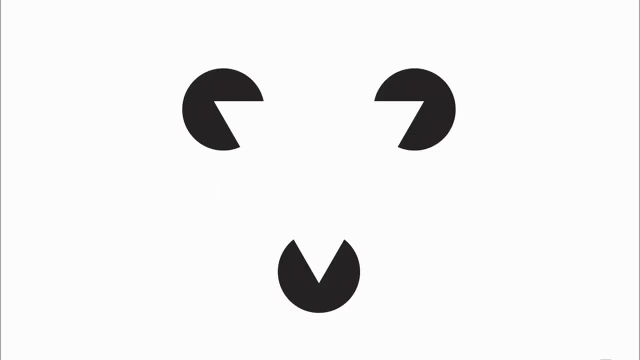 Our brain completes the picture. For instance, in this image, in addition to seeing three Pac-Man or three wheels of cheese, you probably also see the triangle in the middle. That's closure. Or here you have what's known as continuity, where you see the s. 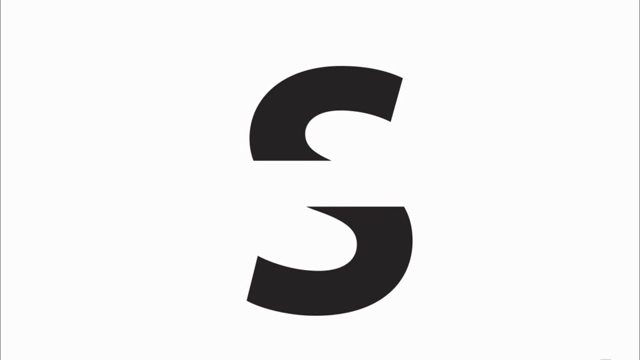 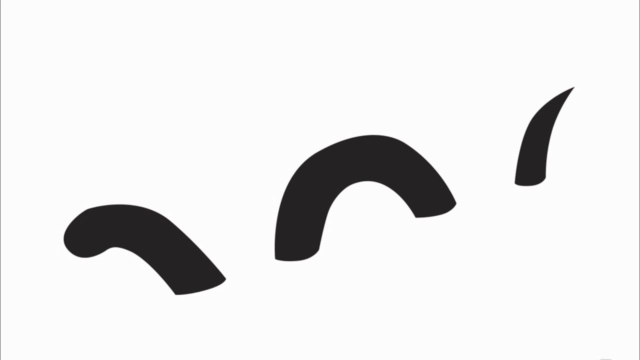 That's closure. you don't just see two random arcs, you see a full s shape. your brain just does that for you. culture can play a role in continuity, for instance here. you don't just see a random sine wave pattern, even though you do end up seeing that full pattern. but what you probably really see is: 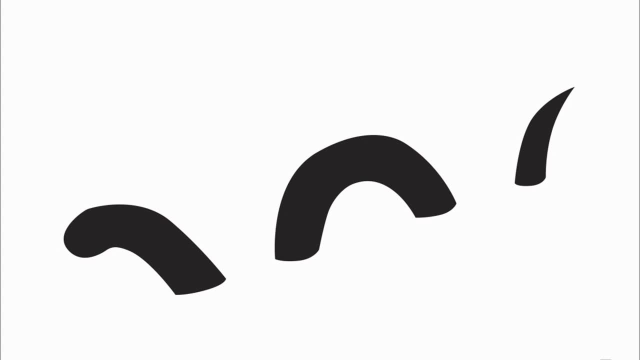 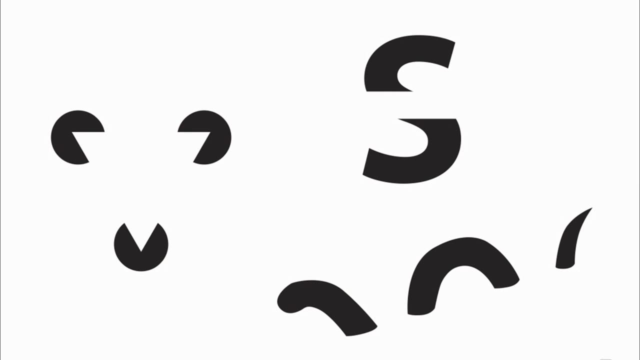 the loch ness monster. that's where culture can have an influence. this isn't specific to visualization, but it's something to be aware of. as you visualize and as you're creating shapes, you don't want them to be misperceived or seen as something unintended by your audience. it could. 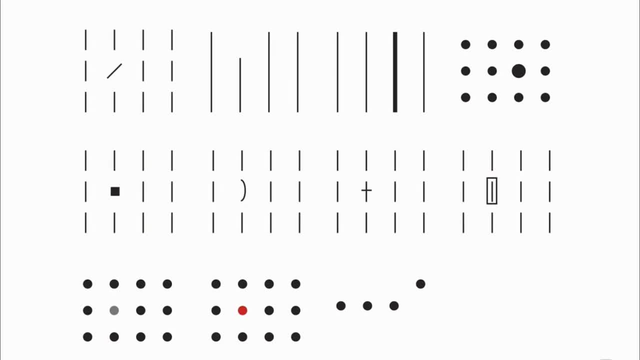 affect how your data is understood. the gestalt principles are key to how people perceive things visually and there are lots of techniques to use to draw the eye understanding how these principles work and to help make your data stand out, whether it's tilting a line or making lines shorter, or 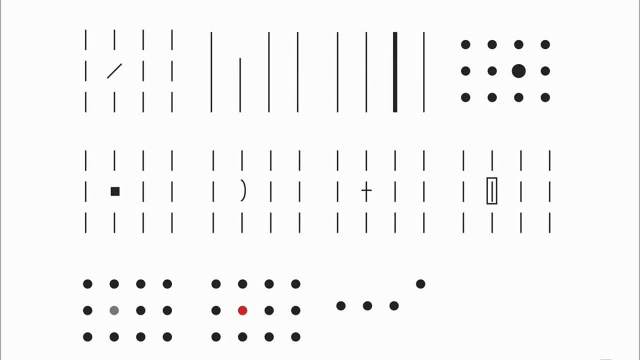 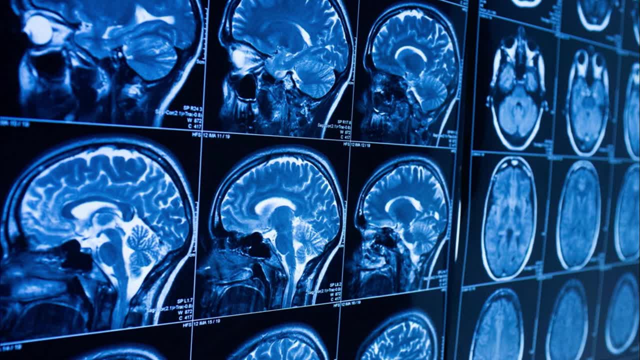 brain scan or every principle for how brains process information. to do a visualization, of course, but knowing it will help designing how to trigger the brain instantly to maximize effect.